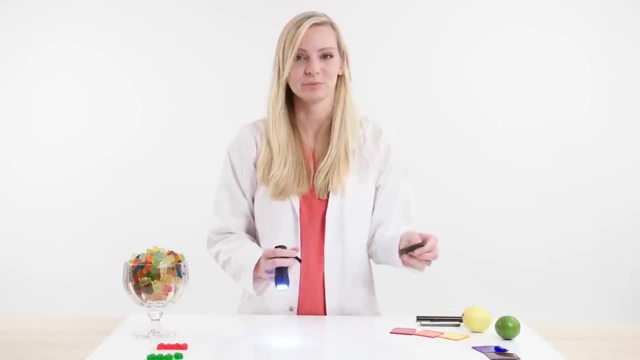 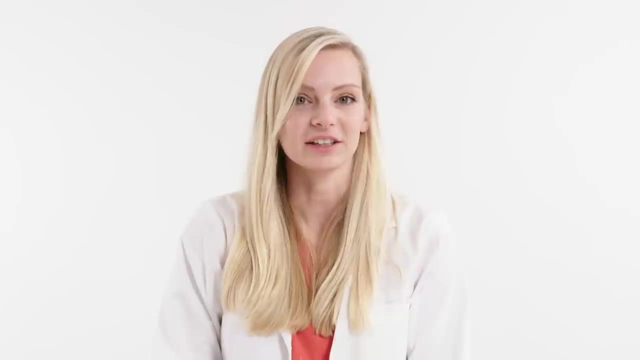 Let's start with this green filter. When we shine the flashlight through the filter, only green light passes through. All of the other colors, including red, orange, yellow, blue and violet, are absorbed, leaving only green to pass through. 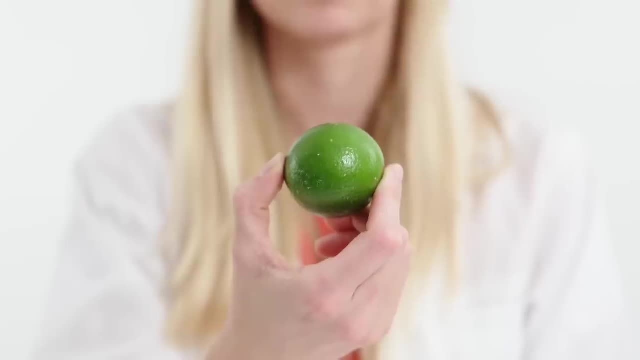 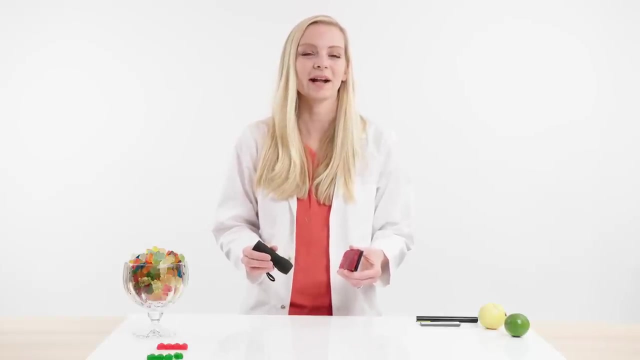 Now let's take a look at this. lime Colors such as red, orange, yellow, blue and violet are all absorbed. Only the color green is reflected, which is why we see that color when we look at the lime. Knowing that filters absorb light, let's think about what would happen if we shined white light. 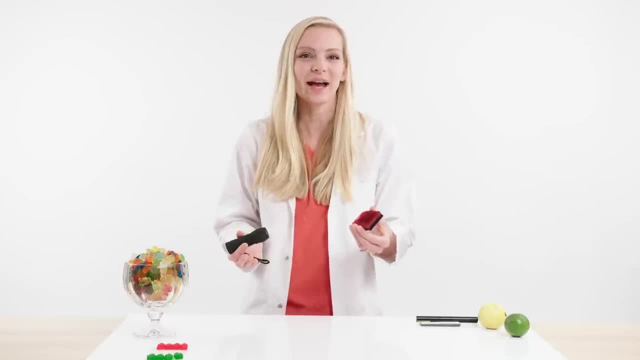 through all the different colored filters. What do you think will happen? Can you take an educated guess? Remember to subscribe to our channel and turn on the notification bell so you don't miss a video. Remember, white light is made up of all the colors of the spectrum. 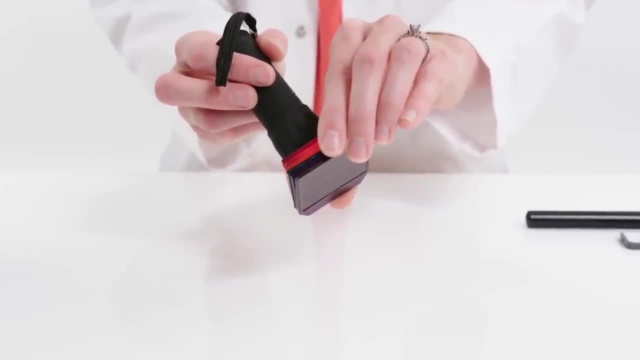 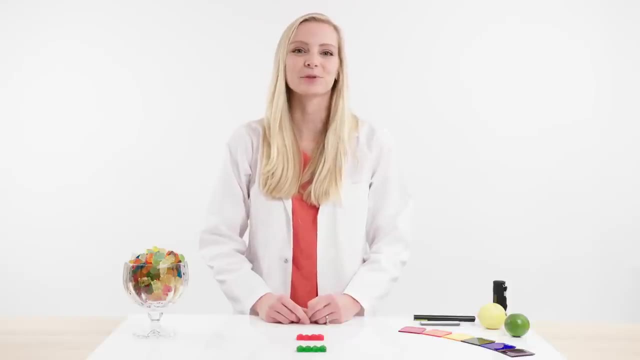 If you guessed that no light will pass through because all of the visible wavelengths of light are being absorbed, you are right. Now we'll have some fun and demonstrate absorption of light using gummy bears and lasers. Here I have a few green gummy bears and a few red gummy bears. 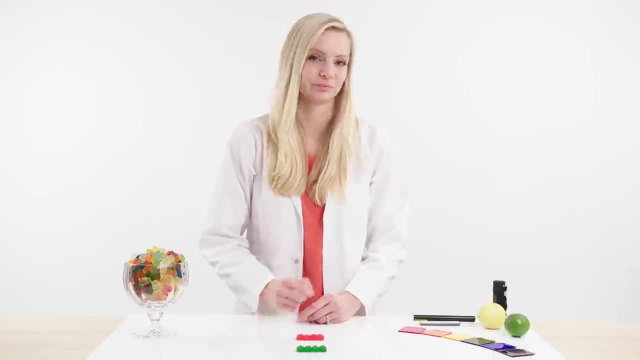 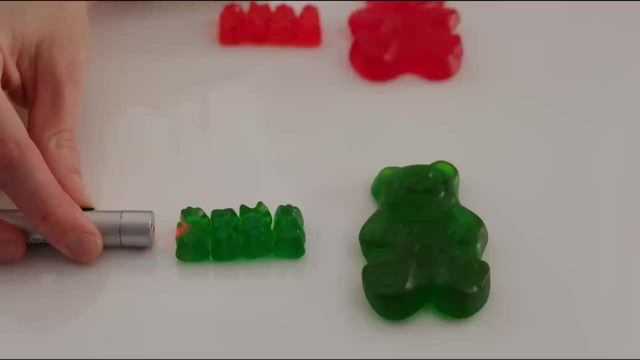 I also have a green laser and a red laser. When I point the red laser through the red gummy bear, the red light passes through. When I point the red laser through the green gummy bears, the light does not pass through. This is because the red light is absorbed by the green gummy bear. 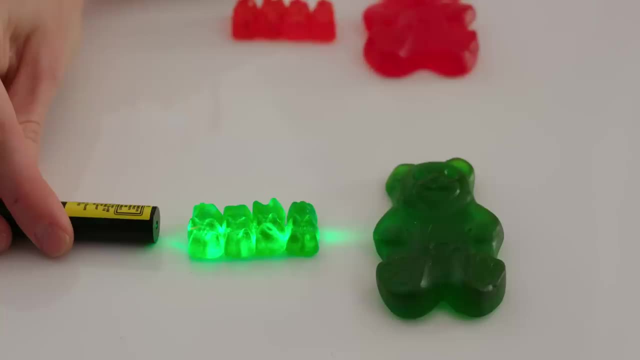 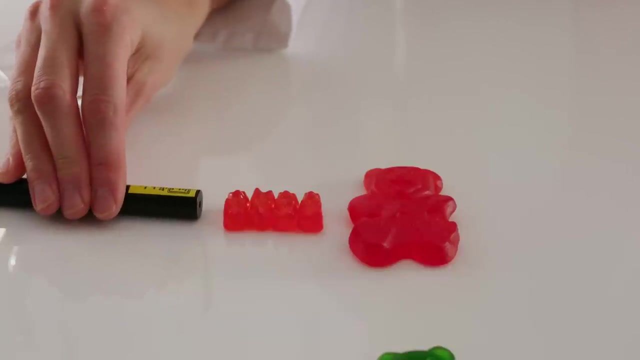 Let's try the same experiment using the green laser. When I point the green laser through the green gummy bears, the green light passes through. When I point the green laser through the red gummy bears, the light does not pass through. This is because the green light is. 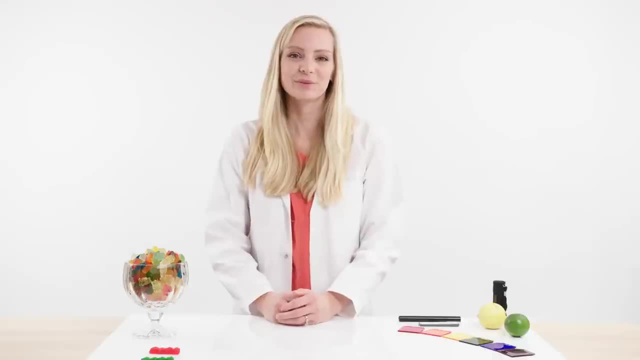 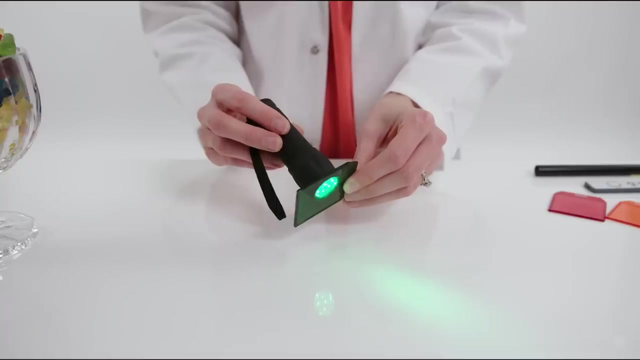 absorbed by the red gummy bear. You can practice your knowledge of absorption of light wherever you go. Just remember that we see objects as the colors they are, because colors from light that you can't see are absorbed, and colors you can see either pass through an object or they reflect off of an object. Check out. 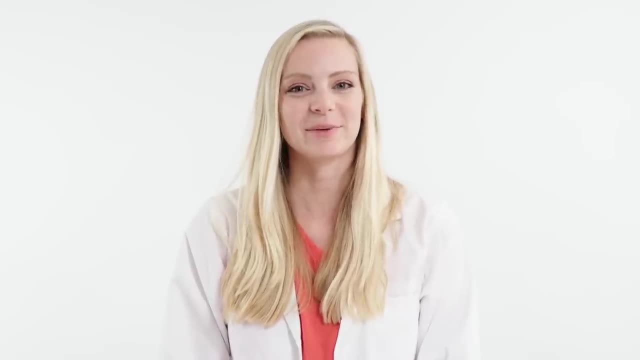 wwwedmundscientificcom for more fun videos and experiments. Thanks for watching.